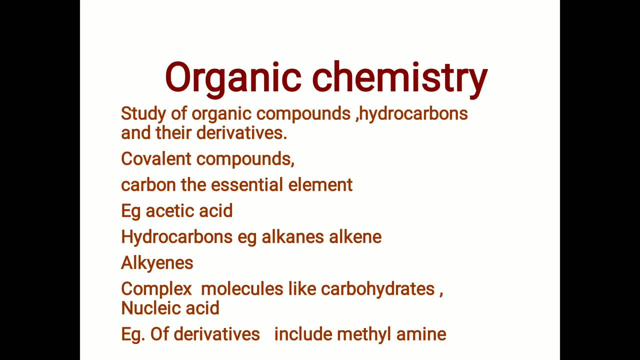 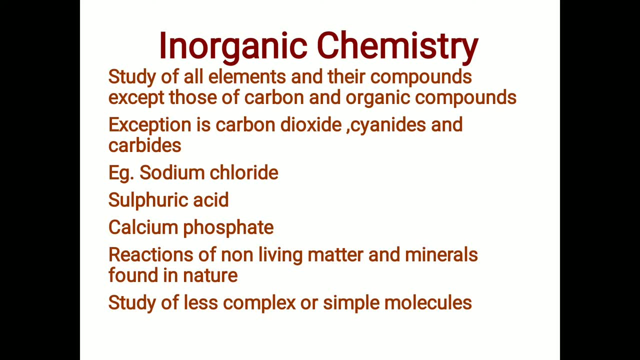 The example of the derivative of organic compounds include methyl amine. Now inorganic chemistry. it is exactly opposite to the organic chemistry. It is study of all the elements and the compounds, except those of carbon and organic compounds. Exception to this is carbon dioxide, cyanides and carbides. 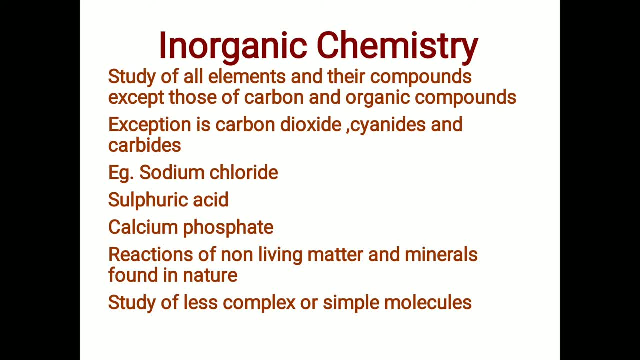 In spite of containing carbon in it, it is studied under inorganic chemistry. The other example of inorganic compounds include sodium chloride, sulfuric acid, calcium phosphate. In inorganic chemistry you study the reaction of non-living matters and minerals found in nature. 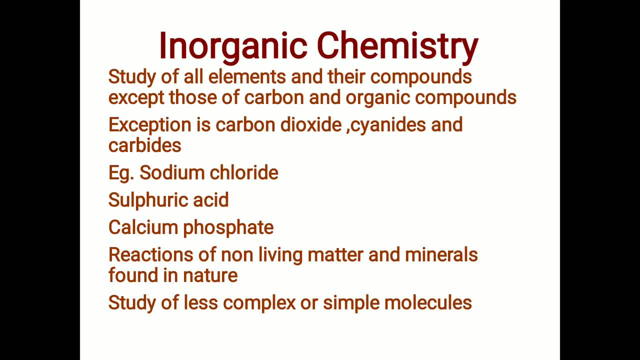 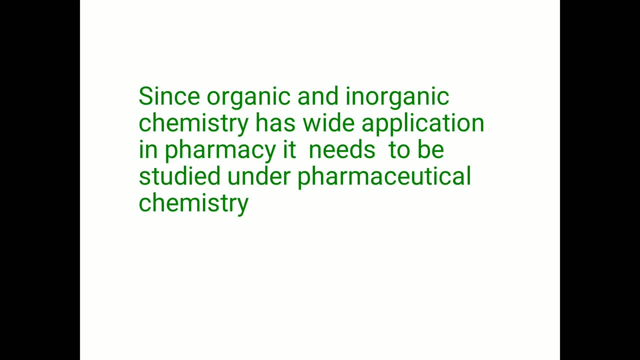 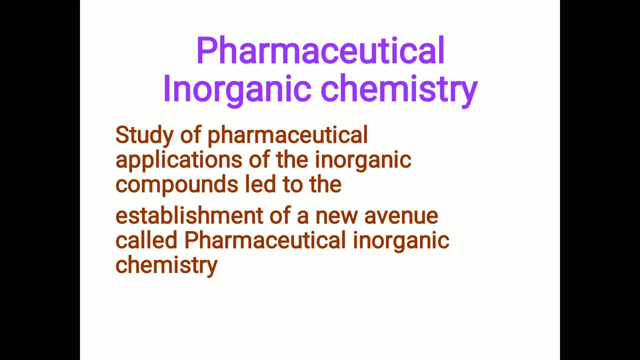 It is a study of less complex or simple molecules. Now, since organic and inorganic chemistry has wide applications in pharmacy, it needs to be studied under the special branch called as pharmaceutical chemistry. Now, what is pharmaceutical inorganic chemistry? The study of application of inorganic compounds has led to the development of new branch called as pharmaceutical inorganic chemistry. 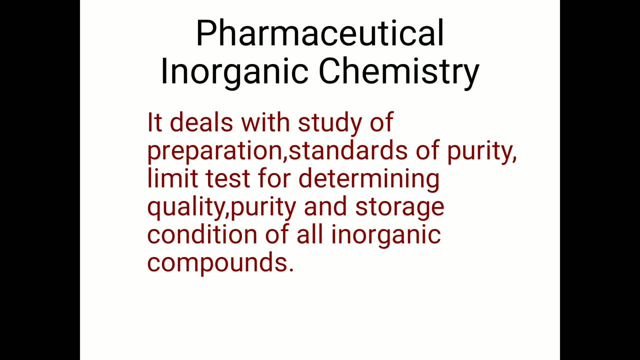 Now let's talk about the definition of pharmaceutical inorganic chemistry. It deals with the study of preparation standards of purity limit test for determining quality, purity and storage conditions of all inorganic compounds. For example, if you talk about sodium chloride, 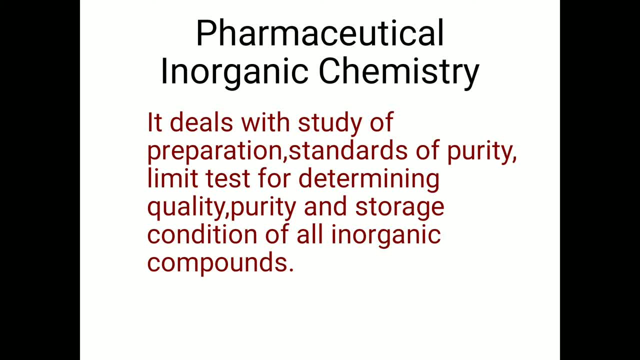 Sodium chloride, which is an inorganic compound. it is used for replenishing fluids in the body. It is studied under pharmaceutical inorganic compounds. Here we study the preparation of sodium chloride standards to maintain the purity of sodium chloride, then limit test for determining the quality of sodium chloride. 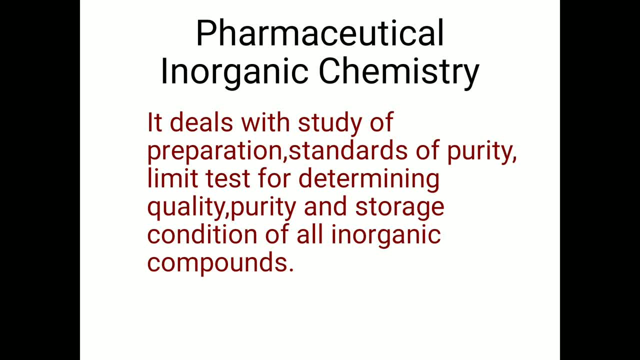 Then what are the purity and storage conditions of sodium chloride? All it is studied under pharmaceutical inorganic chemistry. In the next video let's talk about the applications of pharmaceutical inorganic chemistry. Till then, bye, bye and thank you.